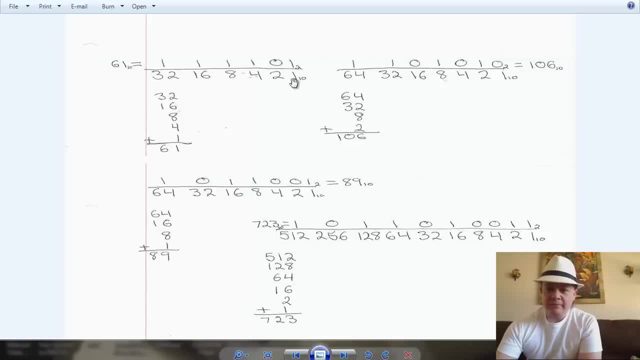 Also, another thing I should tell you too is that When you're going to do places, let's say you're not just dealing with binary. Let's say you're dealing with hexadecimal or octal. You're not going to be just doubling Like 16.. Let's say you've got base 16.. You're not going to go 1,, 16,, 32.. That's not how you're going to do it. 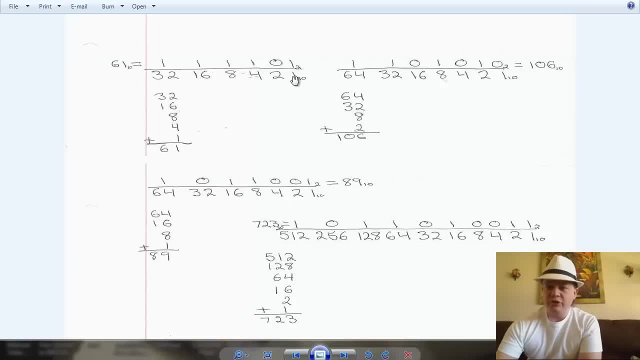 You need to learn. the fundamental of what you're doing here is you're multiplying by 2.. So 1 times 2 is 2.. 2 times 2 is 4.. 4 times 2 is 8.. 8 times 2 is 16.. 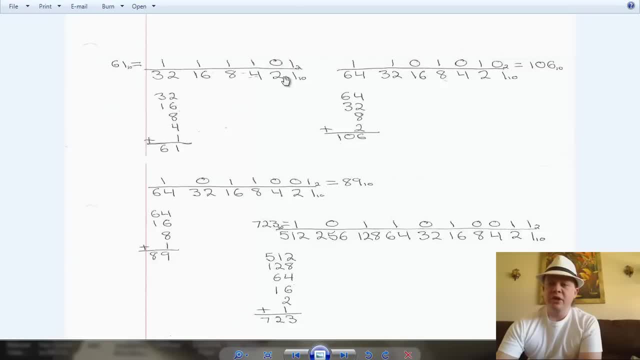 Therefore, if you're working, If you're working with hexadecimal, it would be, you know, 1 times 1.. Well, 1, whatever, 1 times 16, 16.. And then it would be 16 times 16, 256, 512 or something. Anyway, I'll get that tutorial later. 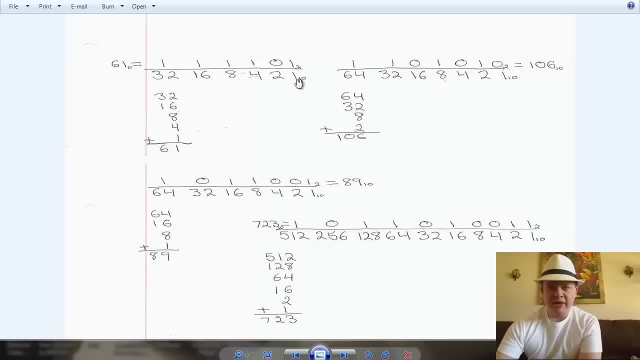 But you have to understand. so we're basically doing multiples of 2.. We're multiplying by 2 for a binary number. So we have 1, 2, 4, 8, 16, 32.. What we're going to do is, every time you see a 1, you're going to be basically multiplying 1 by 2.. 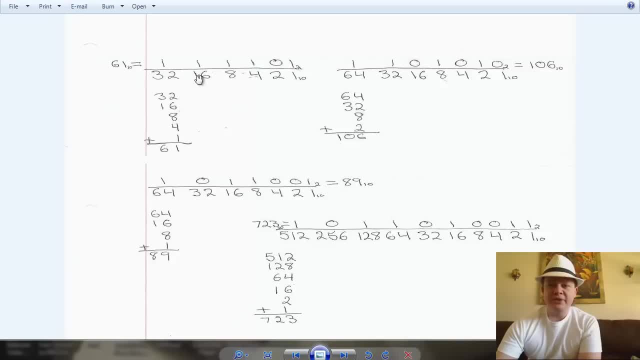 By its placeholder, So 1 times 32.. 1 times 16.. 1 times 8.. 1 times 4.. 0 times 2.. Get nothing out of that. 1 times 1.. That's what you do. 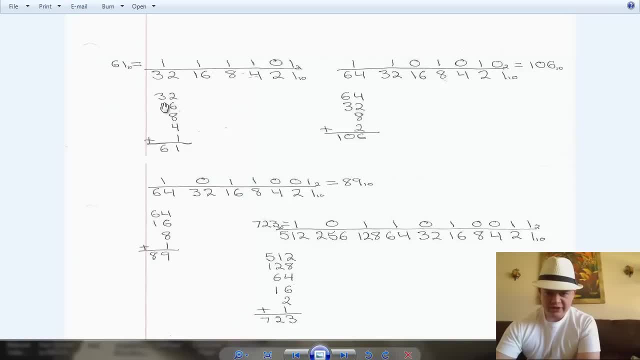 So you see, a 1 here We've got 32.. 1 here We've got a 16.. 1 right here We've got an 8,, 4, 1.. We don't count the 2, because we've got a 0. And we've got this whole column, this row, And we add this up: We've got 61 in decimal. 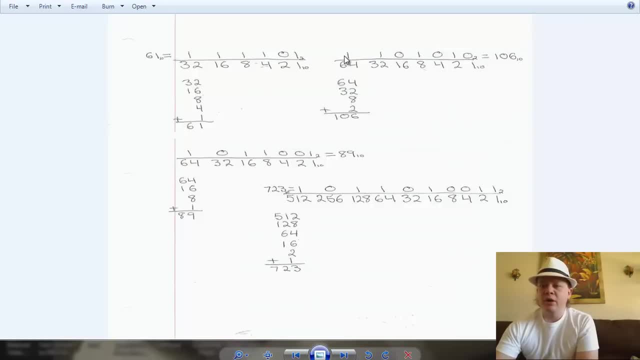 And then let's go to the next problem. We have 1, 1, 0, 1, 0, 1, 0 equals 106 in decimal 64. We've got a 1, so we put 64 down. 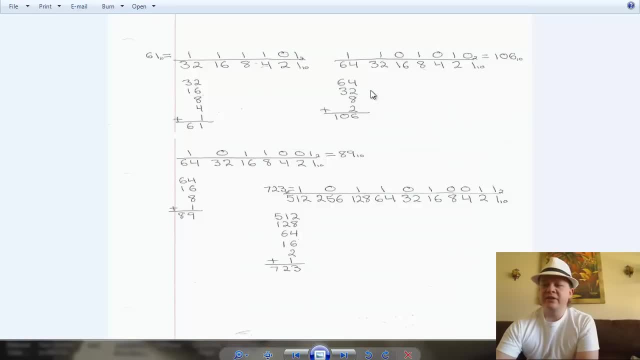 32, yeah, we've got that. 16,. we don't have 8, yes, we do have that. 4, damn phone, sorry about that 4, no, don't have it. 2, yeah, we've got that And 0 for the 1.. No, we don't have that. 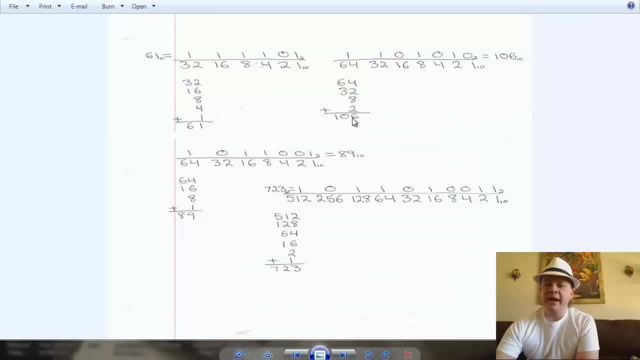 So 64.. 4 plus 32 plus 8 plus 2.. Bam, Right, there you go: 106 in decimal. That's how you convert a binary number to decimal. Now let's get another. look at my wallpaper and go and convert a decimal number back to binary. 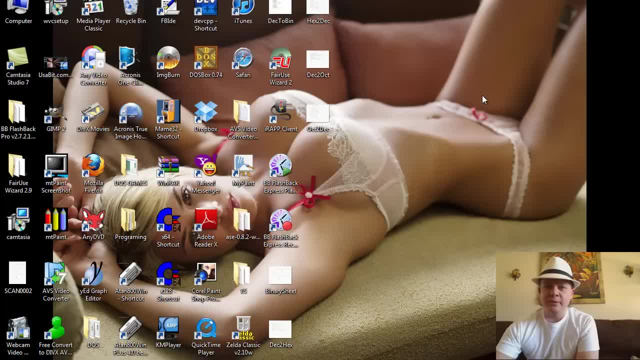 God, I like my wallpaper. I've got a really cool wife, You know she lets me have this kind of wallpaper on here. I'm a lucky guy, I'm telling you I am very lucky. Let's see Decibel 2.. Where have we got it? Decibel of binary. 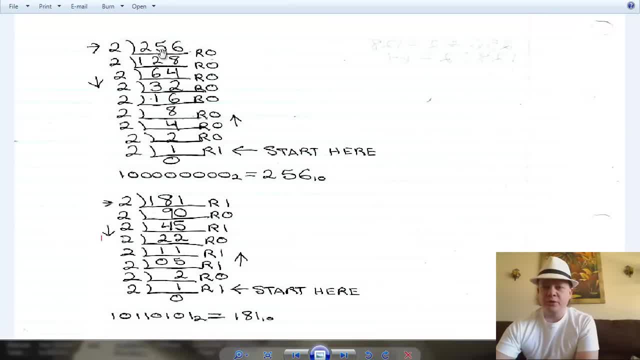 All right, make it a little bigger. All right, let's take the decimal number 256.. Whenever you're going to convert a decimal number into another number system, another weighted number system, you're going to divide it by that number system's weight. 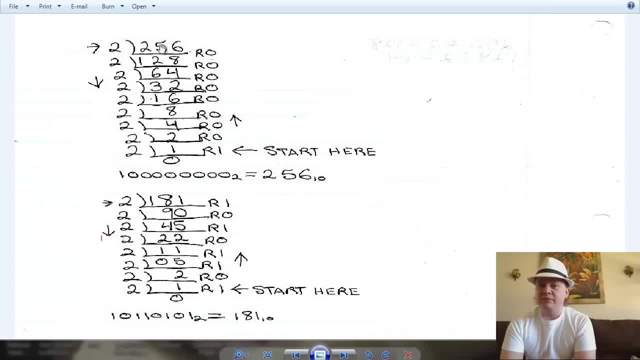 And you're going to take that remainder and that's going to be a digit in your new number, in your converted number. So Now 256,. we're going to divide it by 2, because binary is base 2.. 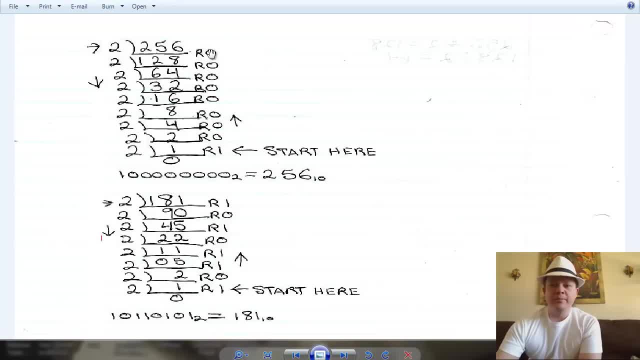 And we're going to have a result of 128 with a remainder of 0.. We're going to take 128, and we're going to divide that by 2. And we're going to get 64, remainder of 0.. 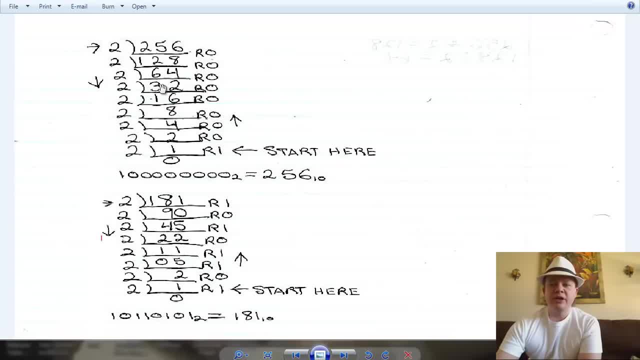 We're going to take 64,. we're going to divide that by 2. And we're going to get 32, and we're going to have a remainder of 0. And we're going to continue dividing all the way down until we can't divide anymore, which is going to be 0.. 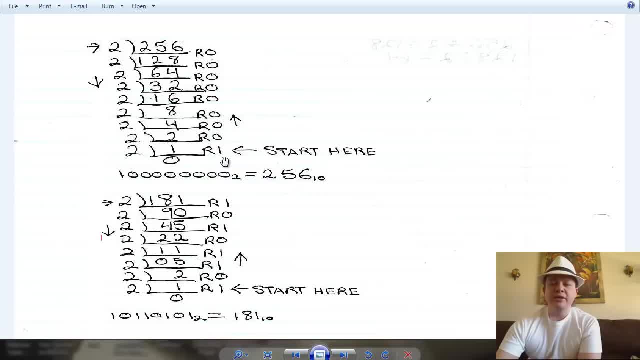 Once we get to the bottom, we're going to go over here to the right And we're going to go- okay, this is where my number, My number, starts from the bottom up, maybe left to right. So 1 here, 1 here, and then we go 0, 0, 0 all the way up. 0, 0 all the way across equals 256, base 10.. 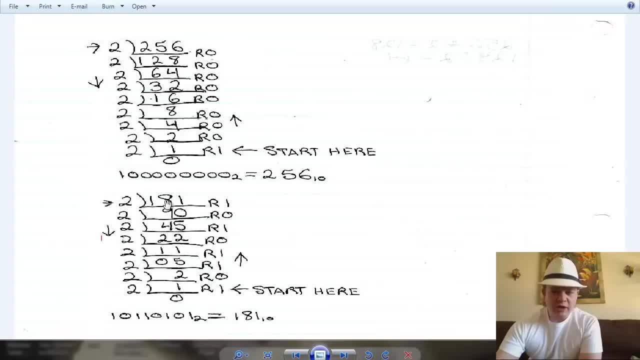 That's it. Let's see here We've got 181.. 181 divided by 2, remainder is 1.. Result: 90.. 90 divided by 2, remainder is 0.. 45 divided by 2, remainder 1.. 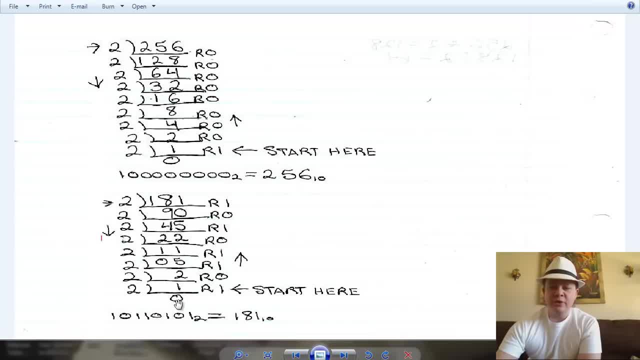 22 divided by 2, remainder 0.. See what I'm saying. We go all the way down. We've got 0. here We go, start at the bottom, work our way up from left to right: 1, 0, 1, 1, 0, 1, 0, 1, 1, 0, 1, 1, 0, 1, 0, 1, you see what I'm saying.